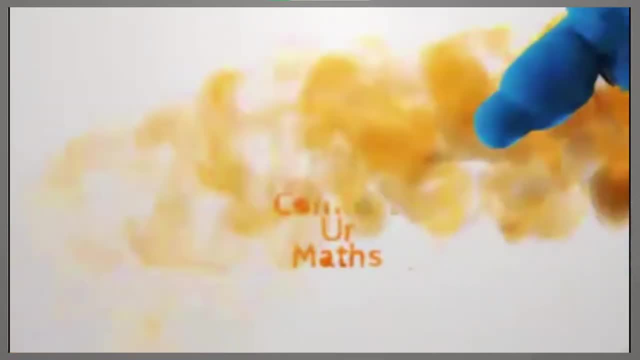 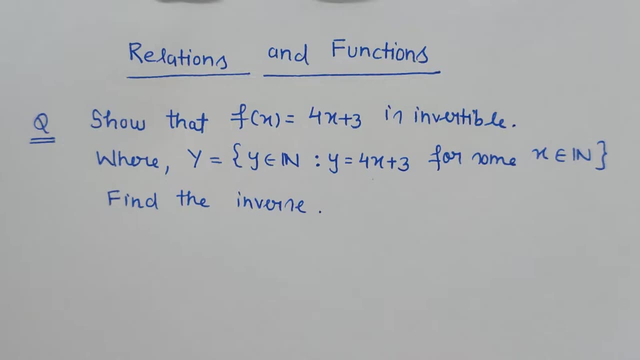 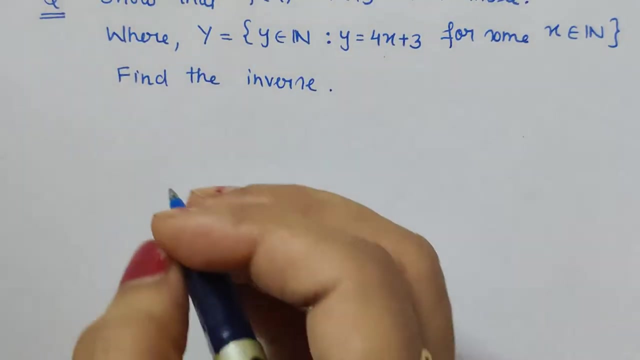 Hello friends, in this video I am going to show how to prove any given function is invertible and then how to find its inverse. So let's see the mandatory condition for proving any function to be invertible. So here the first thing is: function is said to be invertible. 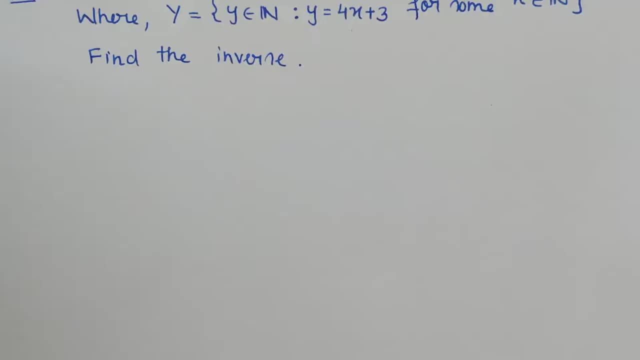 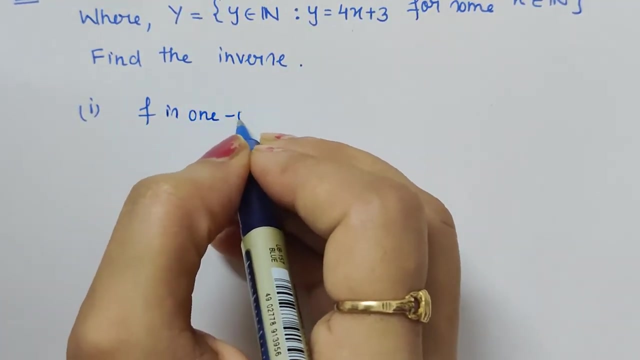 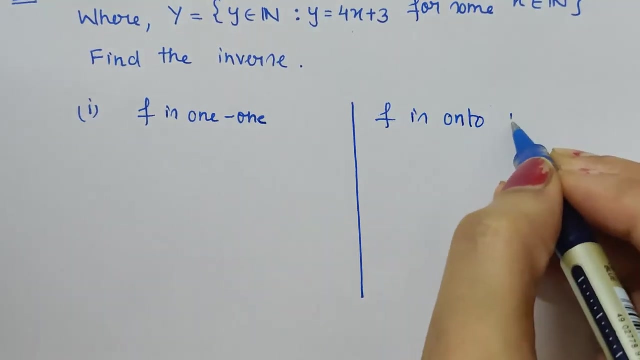 if, and only if, it is 11 and onto. So first we will prove f is 11 and then we will also show f is onto. If we are able to prove these two things, then we can say that the given function is invertible. So for 11, what we have to do- Assume any. 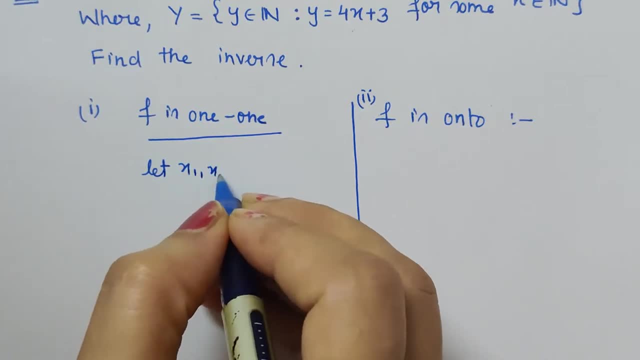 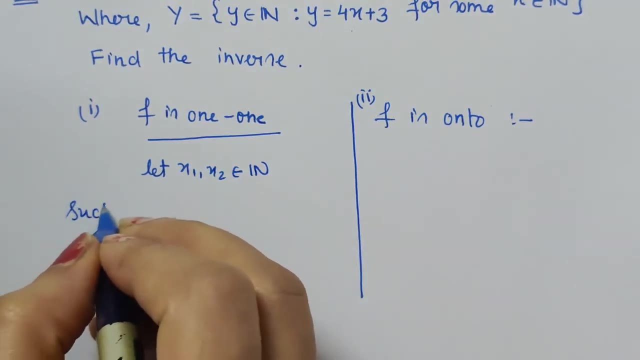 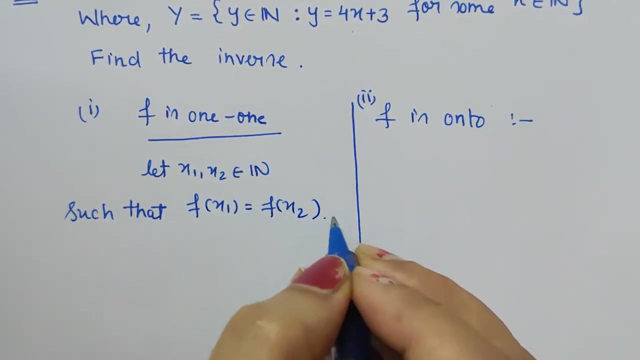 two elements of domain. So let x1,. x2 belongs to the set of all natural numbers and it is the domain given to us, such that f of x1 is equal to f of x2.. Now in the question, f of x is 4x plus 3.. So by putting this in this and this, what do we get? 4x1 plus 3 is 4x. 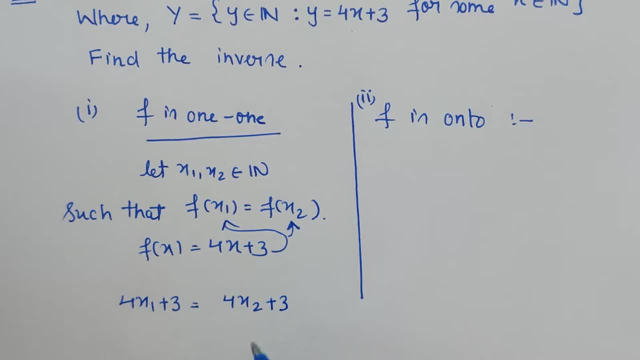 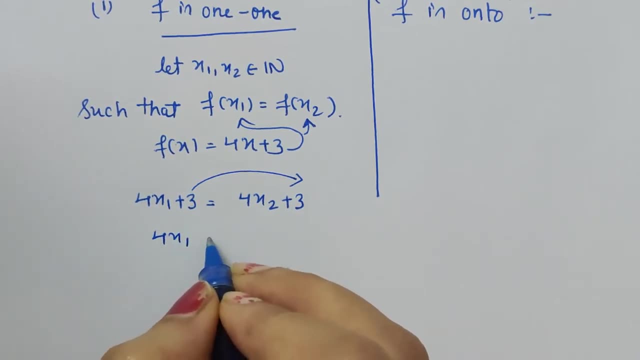 3 is equal to 4x2 plus 3.. Now when we shift 3 to that side, it gets minus 3.. So 4x1 is equal to 4x2, because these two gets cancelled, minus 3 plus 3, and again 4 and 4 gets cancelled. 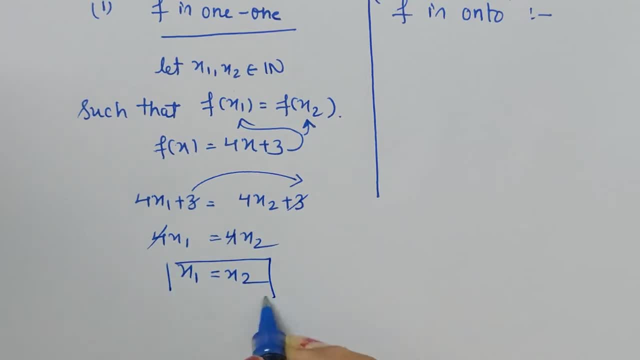 and we are left with x1 is equal to x2, and this is what our objective is: That assuming any two elements of domain such that fx1 is equal to fx2, if we are able to prove that x1 is equal to x2.. 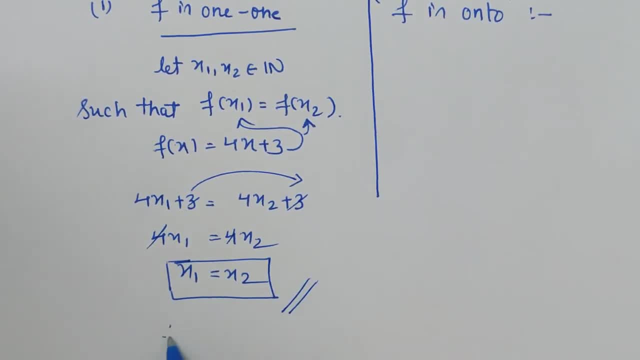 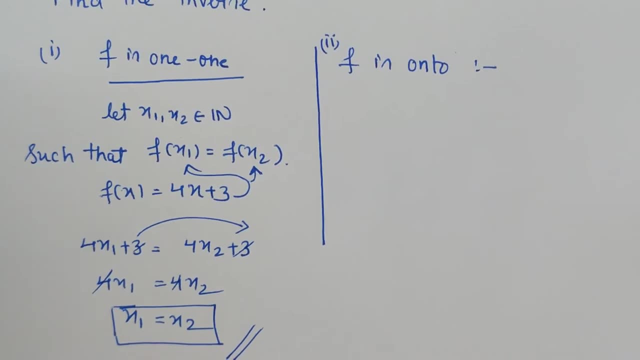 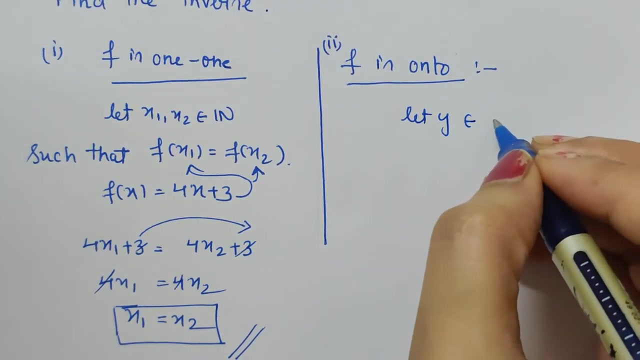 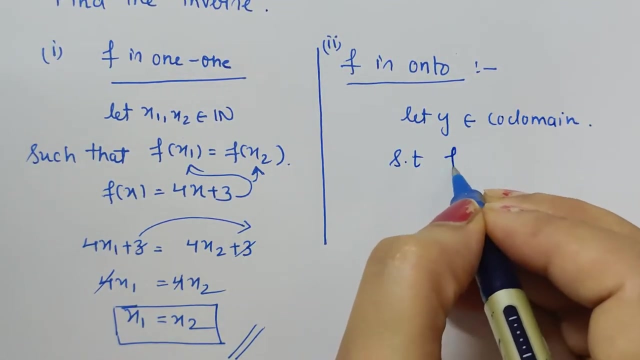 Then it is 11.. So the function is 11.. Now let's see: f is onto. For this we have to assume an element from codomain. So let y belongs to codomain, such that f of x is equal to y. This we have to show. 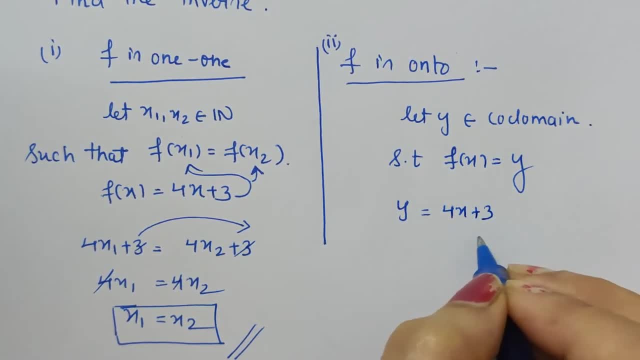 What is y given to us, It is 4x plus 3.. Now we will write x in the form of y, So it can be written as: x is equal to y minus 3 upon 4.. At this step, under onto function proof, 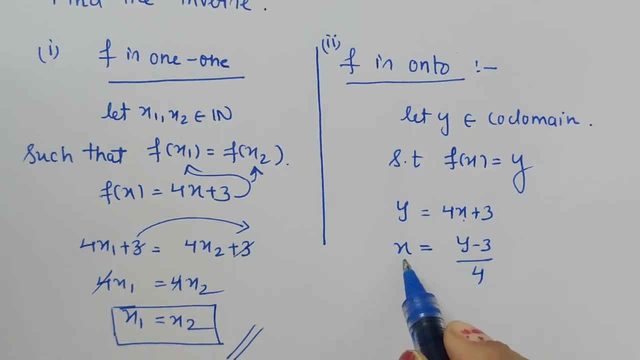 we have to check that for every y x exists or not. So here for every y means we have to consider all those elements which belong to the codomain and for that, whatsoever result get should belong to domain. so here in the question: what definition is given to us for? 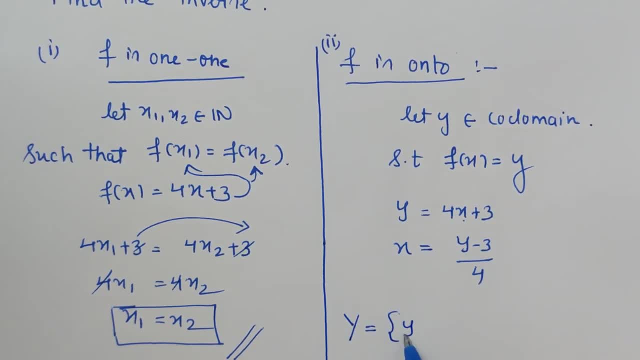 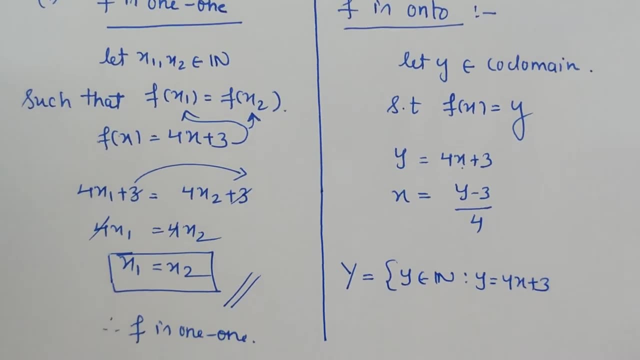 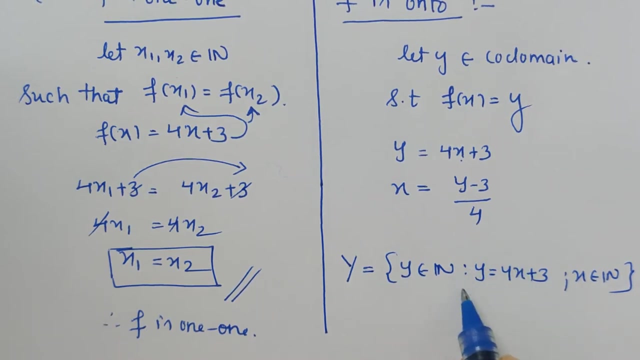 codomain. codomain is the set of all natural numbers, such that 4x plus 3, such that it is 4x plus 3 where x is any natural number. that means y is the collection of all result obtained solving this equation, and here x to be taken from natural number. so the first natural number. 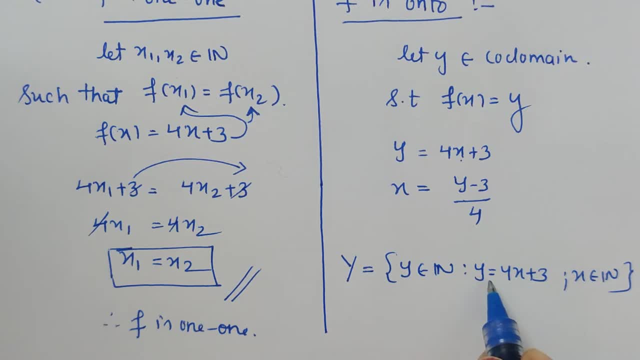 is 1. so if i put x equal to 1 here, value of y is 7. that means the value of codomain begins from 7 and all larger numbers. so here, if i start putting 7, 7 minus 3 is 4, x will be 1, isn't it? so it 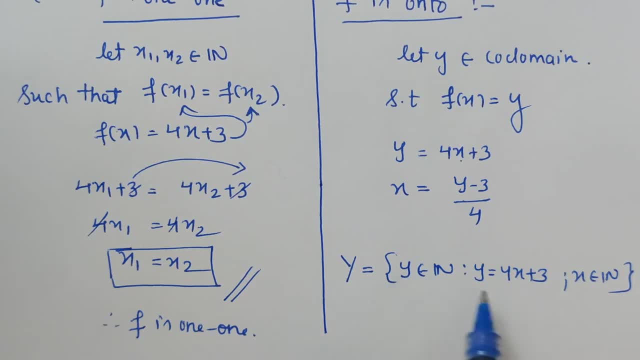 satisfies. so i started with putting the smallest value of the codomain and since x exist for that value and for those values in domain, therefore we can say the function is codomain onto. so here x is y minus 3 upon 4. so here what we have to state for every y in codomain: 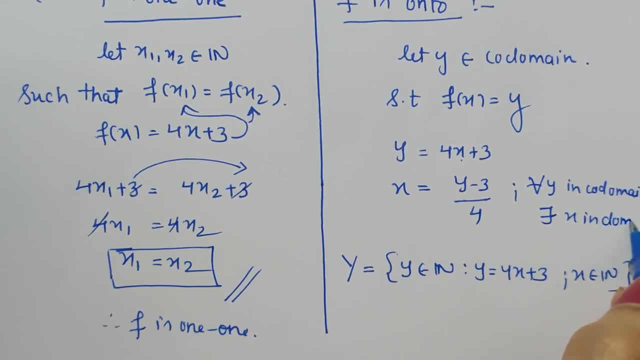 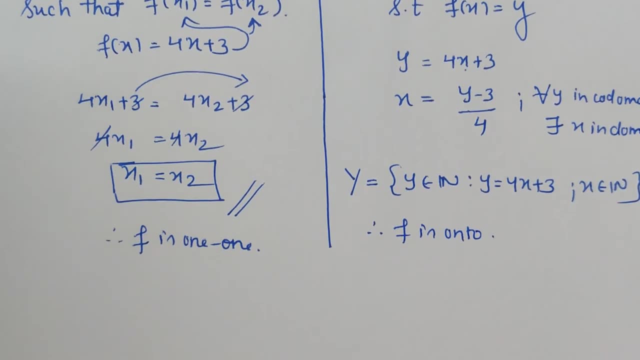 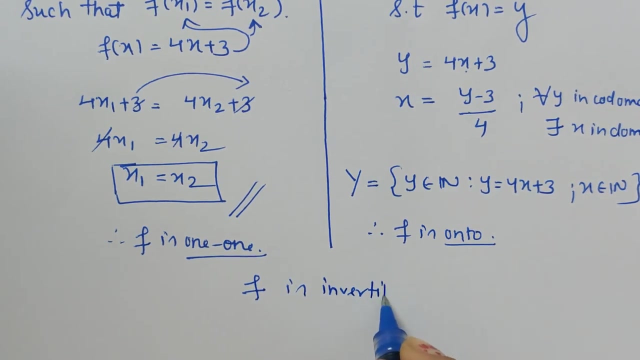 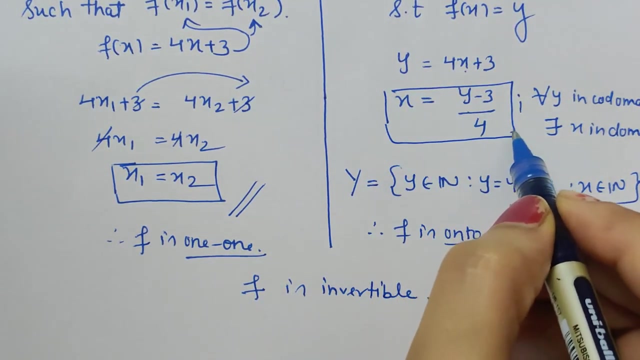 there exists x in domain. this we have to write. therefore, the function is onto, and when the function is 1, 1 as well as onto, we can say that f is invertible. the given function is having its inverse, and what will be the inverse whatsoever? we have written x in the form of y. that is the inverse, actually, but in the